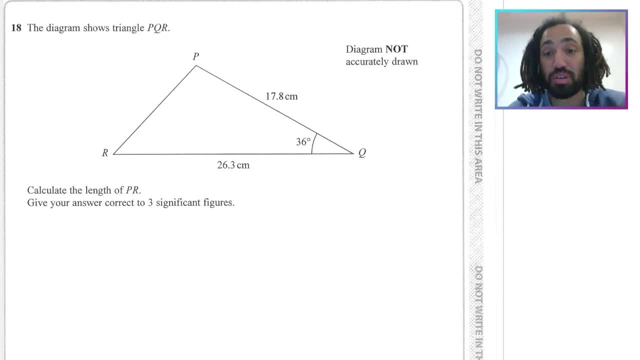 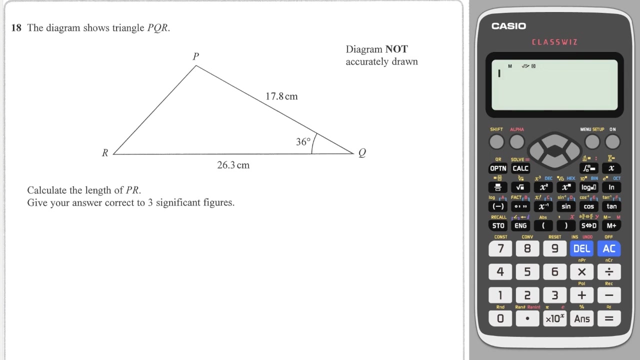 Hello, my name is Mr Asprey and this is number 52 in my IDCSE exam question series, and this is sine and cosine rule. If you do find it useful, please do like the video and let's get into the maths. Okay, question number one is a straightforward question where you need to find 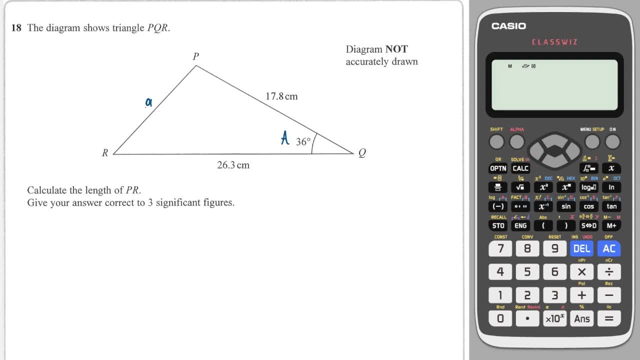 this side I'm going to go with little a, because then I can label the angle capital a and I've got the two sides either side the angle. so this is going to be the cosine rule. So I can write that a squared is equal to the two opposite sides, or, sorry, the two other sides squared minus two lots. 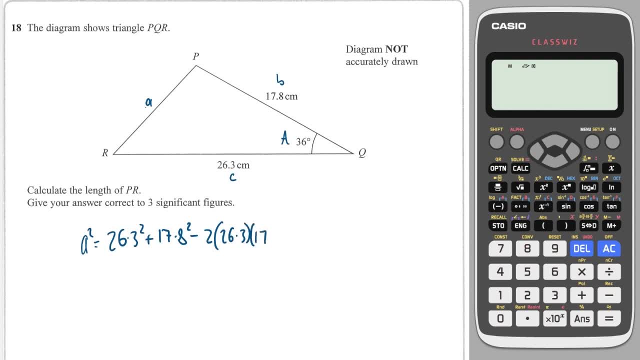 of the other two sides multiplied together, multiplied by cosine of 36.. So we go to our calculator and we do two point sorry, 26.3 squared plus 17.8 squared minus two times 26.3 times 17.8 times cosine of 36. 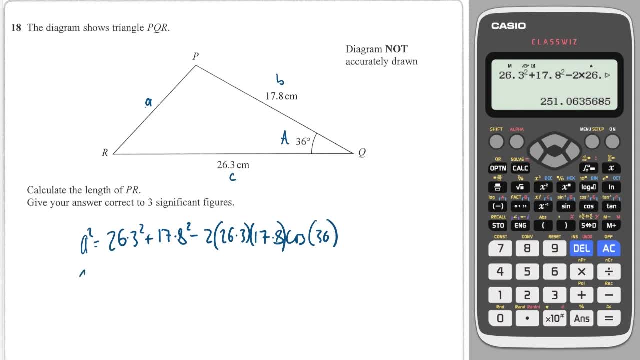 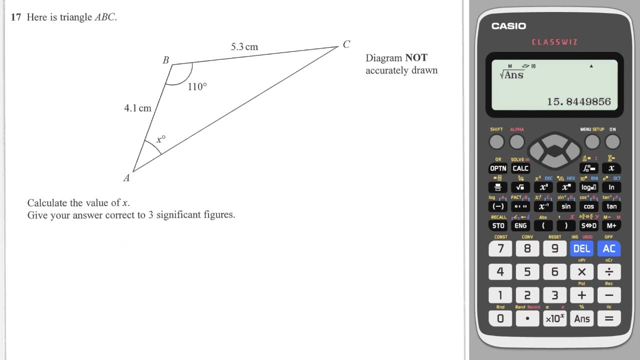 close brackets equals 251.. We write that down so the examiner knows what we're doing, and then we square root that to get our value and we press square root answer and it's 15.8.. Okay, next question: we are looking for the angle. 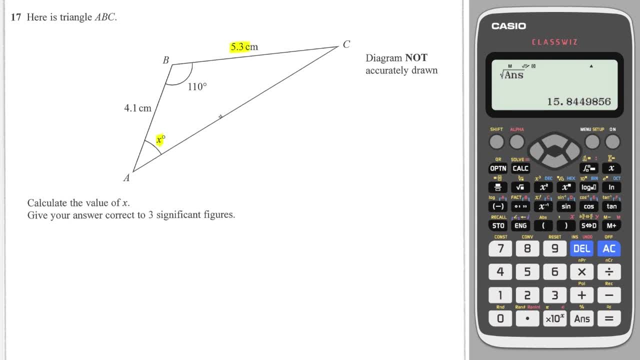 X. We have its opposite side, but we don't have an angle and its opposite side given to us. and if we don't have that, that means we'll use the cosine rule. So we're gonna use the cosine rule to work out a, and I'll call this one the angle opposite, and I will do that by. 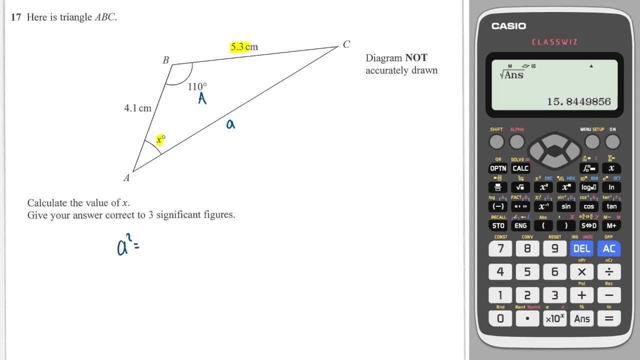 doing squared is equal to again, 4.1 squared plus 5.3. squared minus 2 times 4.1 times 5.3 times cosine of 110.. I'll put that into my calculator. Press equals: I'll square root the answer. 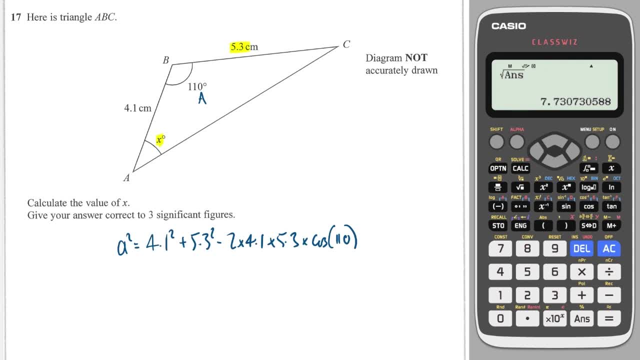 and I'll get 7.7.. So now this is 7.7.. So now I do have an angle and it's opposite pair, which means I can use the sine rule. Just write here: a is equal to 7.7.. 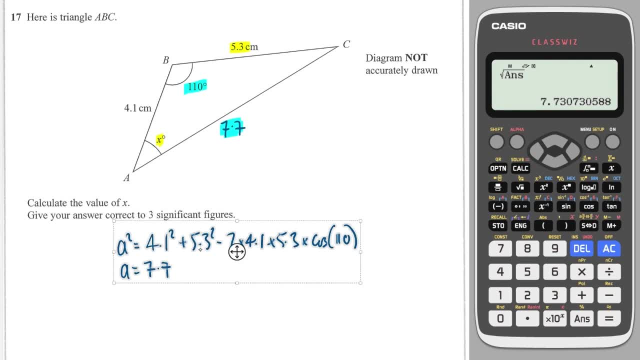 So, using the sine rule, this tells me: the sine rule states that sine of the angle over its opposite side- 5.3, is equal to sine of another pair again over its opposite side. Okay, I can rearrange this by multiplying both sides by 5.3. 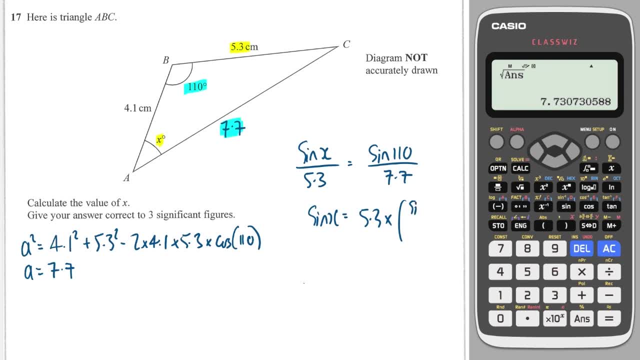 So I get 5.3 times by sine of 110 over 7.7.. So you put that into our calculator: 5.3 multiplied by sine of 110, close brackets over the last answer. It's better than writing 7.7.. 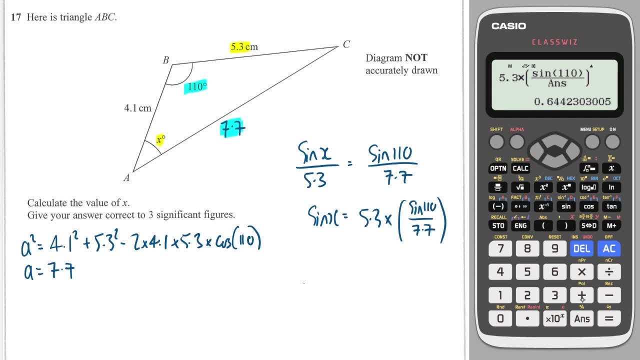 And that equals 0.644.. So sine x equals 0.644.. So therefore, x is equal to inverse sine of 0.44.. And we press shift: sine of that last answer equals, and it's 40.1 is our angle. 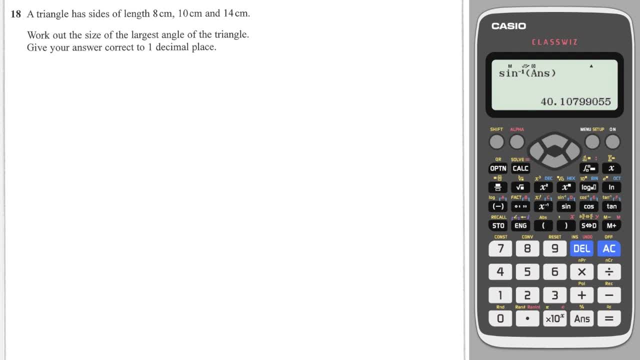 Okay, next question: we've got a triangle with no diagram- How stingy. And it says: work out the size of the largest angle. So if I were to draw this, let's call this side, the largest side, 14.. And then we've got 10 there and let's say 8 here. 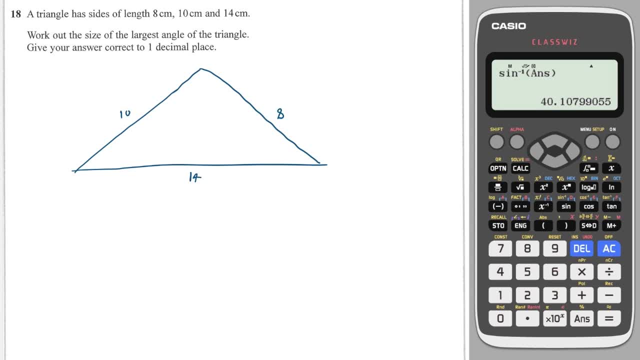 Then the largest angle will be the one opposite the largest side, Because if you think about it, 14 is the largest side, So it spreads the other two sides out the furthest, So this is going to be the longest side. So I'm going to call that one capital A. 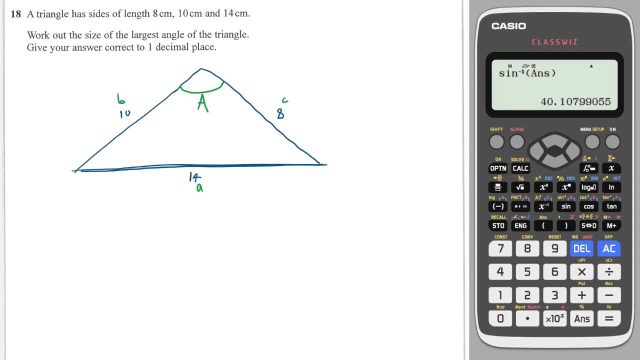 This one little a, which means these two could be b and c. Okay, now you're not given the cosine rule for angles. You are given the cosine rule for a side which looks like this: So what I would do would be to take this big chunk here. 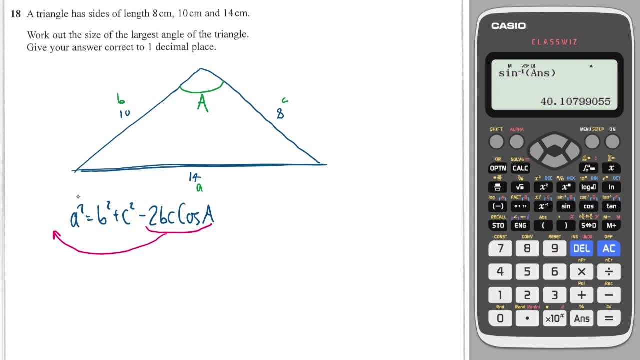 and add it to the other side and then take a squared and subtract it to this side And that will give you two b c. cosine capital A is equal to b squared plus c squared, minus a squared, And then you can get cosine a by dividing both sides by two b c. 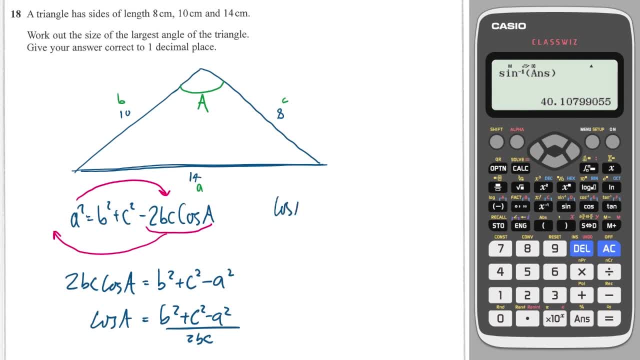 So now I can sub those values in. So I get: cosine of a is equal to 10 squared plus eight squared minus 14 squared, all over two times 10 times eight. So in my calculator I'll press the fraction button first. 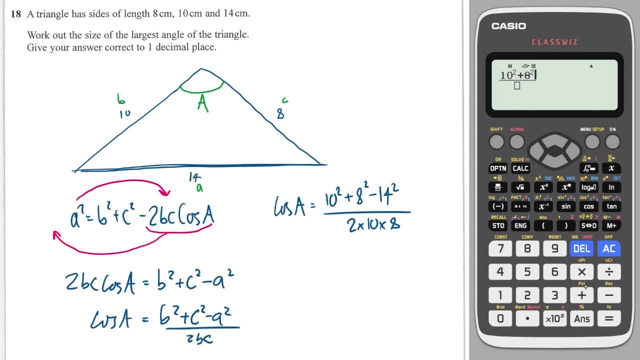 I'll do 10 squared plus eight squared, minus 14 squared, all over two times 10 times eight, and I'll get minus 0.2.. And then I will work out F plus eight times eight by doing the inverse cosine of that value. so I'll do shift cos of the answer. 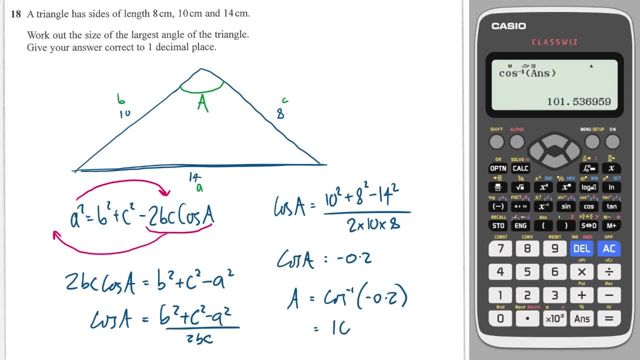 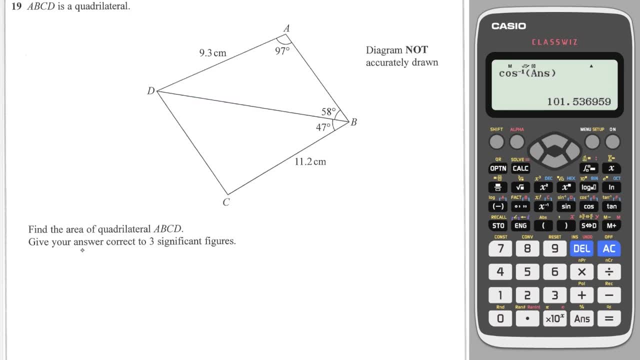 and I will get a hundred and one point five. perfect, okay. next question: I'm asked to find the area of the whole quadrilateral. so first we just bought. as you've got a triangle here with two angles, which means straight away you can work out the third by taking away 97 and 58 from 180 to get 25. so now that's. 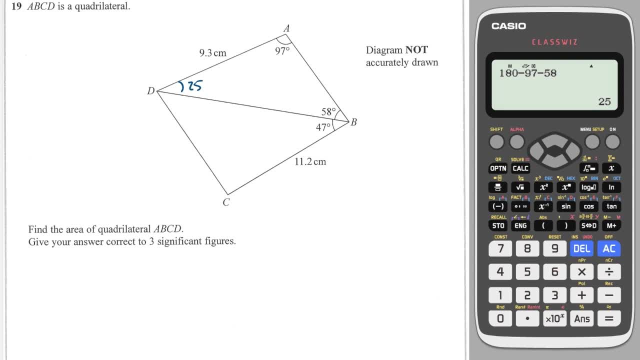 helpful because you have a. actually it's not that helpful, but you've got. you've got a pair here, which is helpful means you can use the sign rule, which means from here I can work out this side, which is going to be very helpful because that's in. 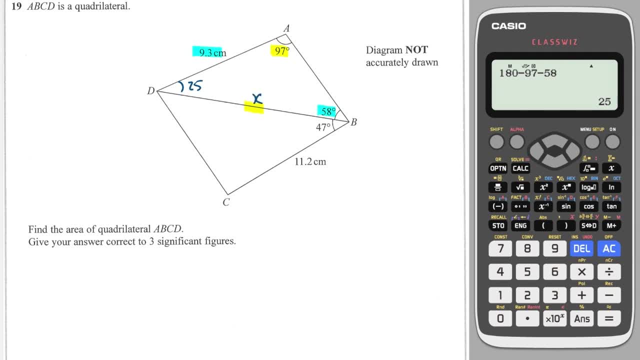 both triangles. okay, yeah, we've got there in the end. actually, let's call that X. so X over sine 97 is equal to 9.3 over sine of 58. so X is equal to our calculators. we would do 9.3 over sine 58 and then we would need to. 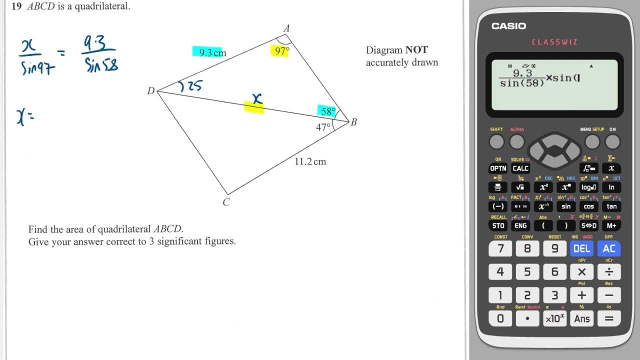 multiply that by sine 97, right, exactly 10.88. okay, now I know 10.88, I can work out the area of both triangles, because all you need to work out the area of a triangle is two sides and the angle in between them. I had twenty five was useful, so that's a half. 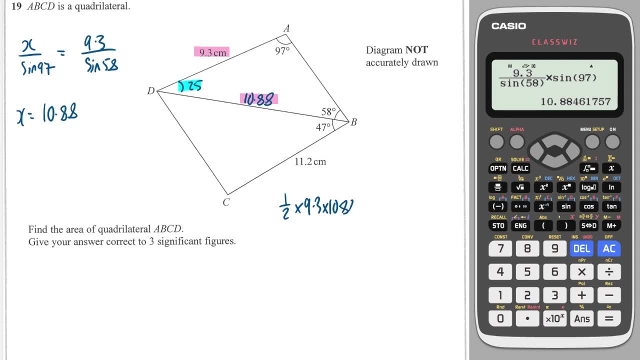 times nine point three times ten point eight, eight times by sine of 25. that's the formula which is given in your formula sheet. so we will do a half times nine point three times by the previous answer times, by sine of 25, and this will give us 21.4 or 21.39. and then let's look at the other triangle. well, we've 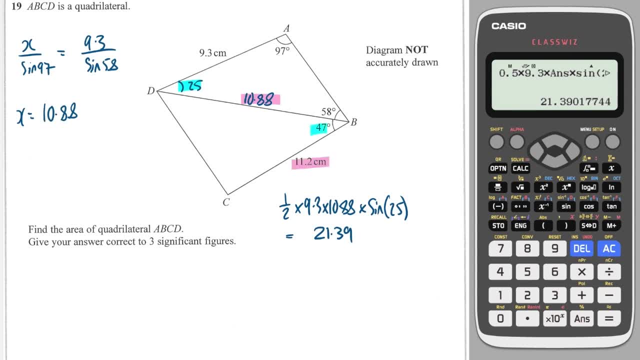 got two sides and we have an angle in between them. so we can do the same thing, we can work out the area of that triangle so that one is 11.2 times ten point eight, eight times by sine of 47. so we do zero point five times eleven point. 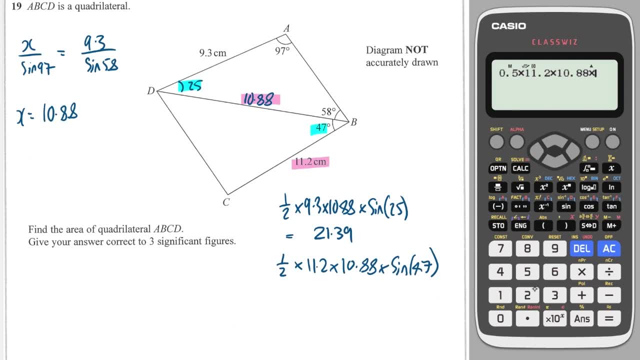 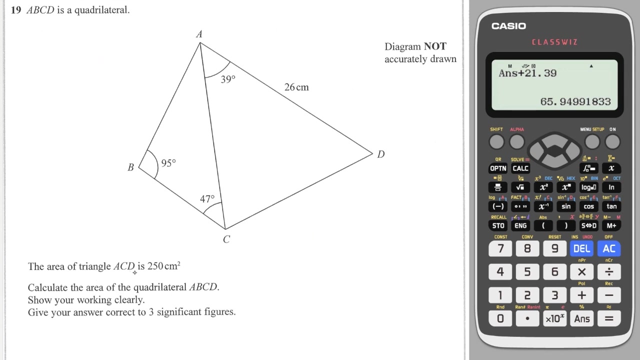 nine times by ten point eight, eight times by sine of 47, and this gives us 44.56. so we add that to our 21.39 to get the total area of ABCD, and that's equal to 65.9. okay, we've got another question here, but this time you're given the area of a CD, so in here. 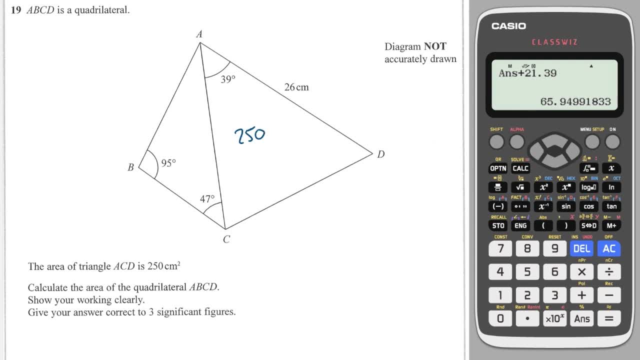 is 250, so we can use the fact that you need two sides at an angle in between to work out the area. so let's call this one X, so the area formula will be: 250 is equal to one half multiply 1 by 1, plus the миллиonhour of a 10 to n over x, and we've got. our value is that, and then 하겠습니다. 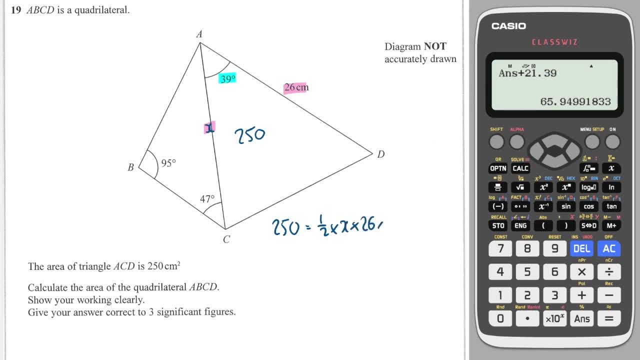 so x order and we're going to get 9.. breaks between five and 7يتhe onlyコ you return and multiplied by x, multiplied by 26 times by sine of 39.. Okay so, in order to work out x, I will need to. 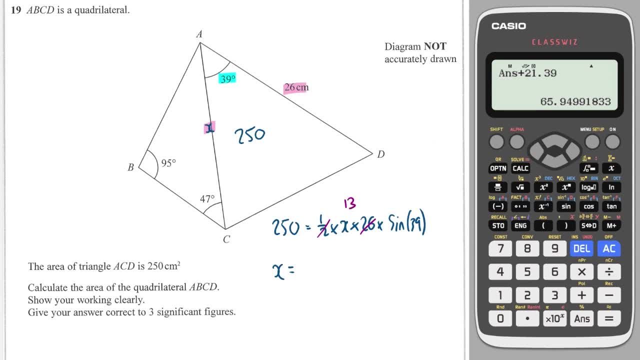 well, first, what I can do is a half times by 26 is 13.. So I'll divide by 13 and sine 39. So it'll be 250 over 13 sine 39. So I'll do 250 over 13 sine of 39,. 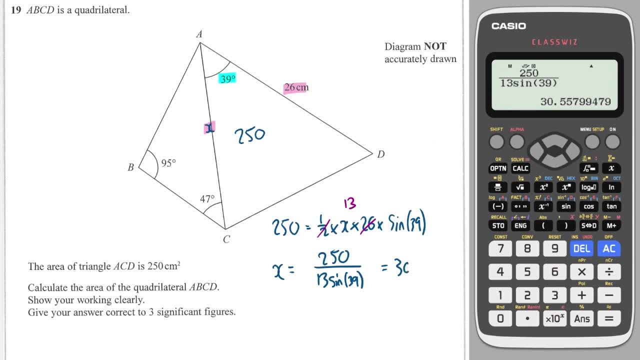 and that will give me 30.56.. So that's my value for x: 30.56.. And I need to work out the area of the quadrilateral. Well, at the moment on the left side, I've only got one. 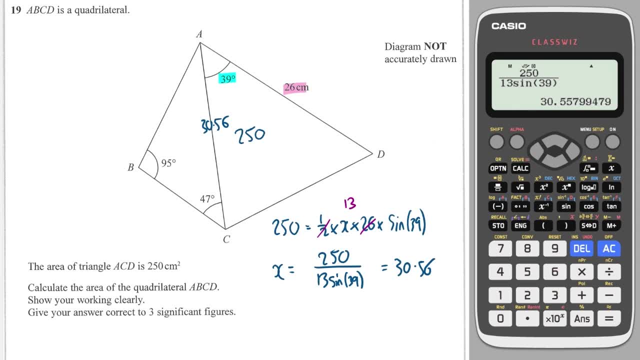 I need one side, I need two sides. So what I can do is I can use the sine rule, because we have a side and we have its opposite pair angle, So I can use that to work out this side here which is opposite this angle here. 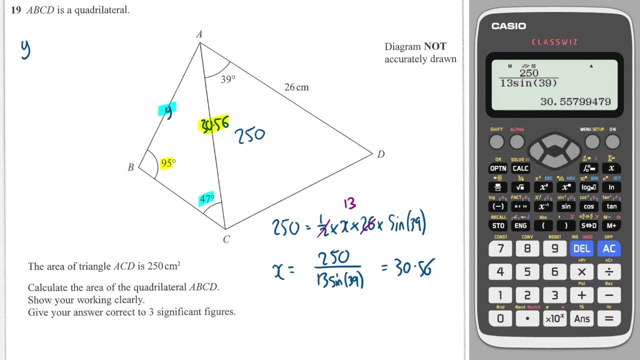 So let's call this one y and I can say that y over sine 47 is equal to the pair that I have, which is 30.56 over sine of 95. And then I can work out y on my calculator by doing this answer over sine of 95,. 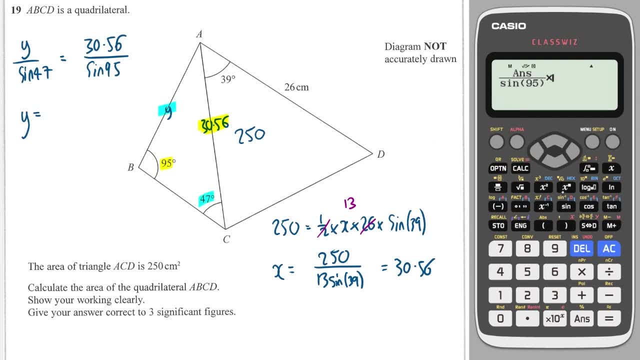 and then multiplied. So I'll bring the sine 47 up to the other side and that will give me y, which is 22.43.. Okay, so 22.43, and now I can work out a area, as long as I have two sides and the angle in between them. 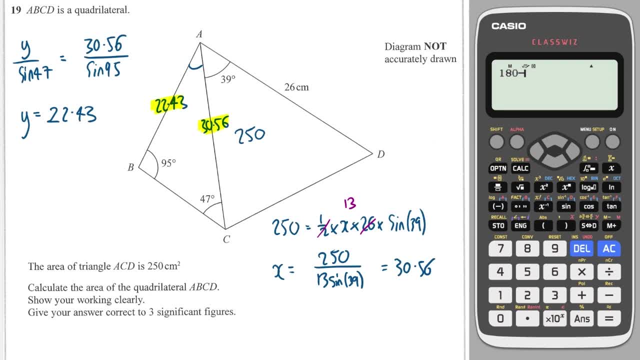 And the angle in between them I can work out because I know two of the other angles in natural in that triangle so I can take them away from 180 to leave me 38 up here. So the area of this triangle ABC is equal to 1 1⁄2 times by the two sides opposite. 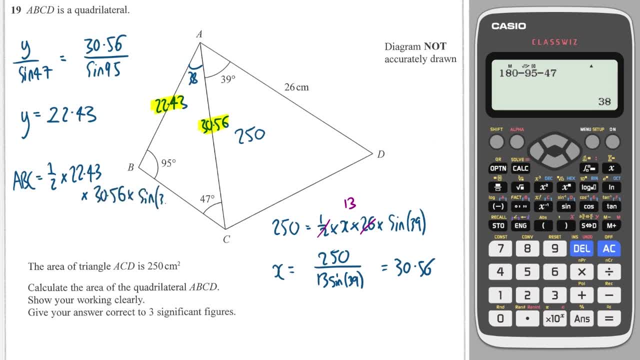 one another times by sine of the angle in between them. So I will do 0.5 times by 22.43 times by 30.56 times by sine of 38, and I'll get an area of 2 1, 1.. 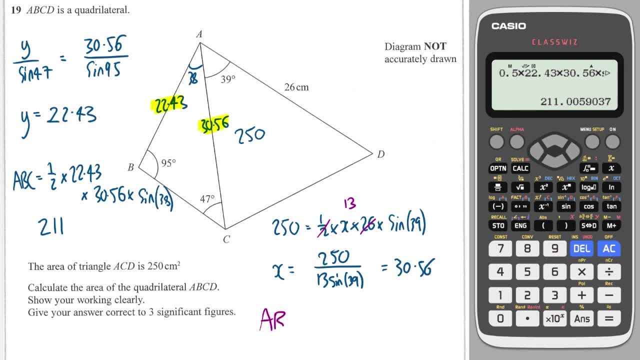 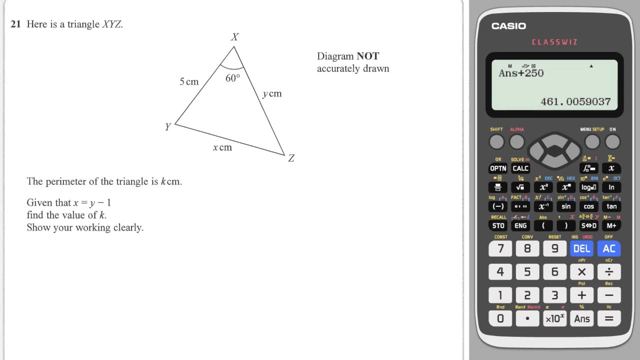 So the total area of quadrilateral ABC is 2: 1, 1 plus 250.. Which is 461,. perfect, Okay, tricky question alert. We're asked to work out the perimeter of the triangle and it says that, given that x is equal to y minus one, 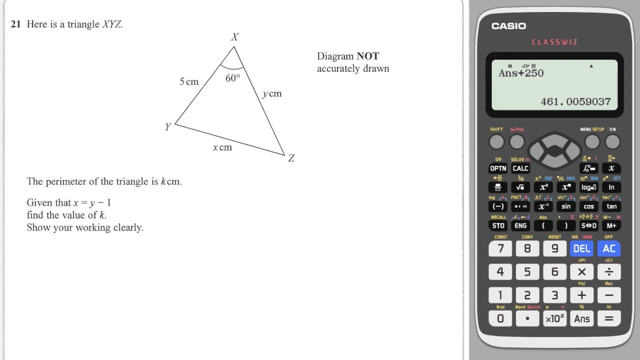 find the value of k. Well, if x is equal to y minus one, then y is equal to x plus one, and I could write that over here: is x plus 1. and now I have one angle and I have an expression at least. 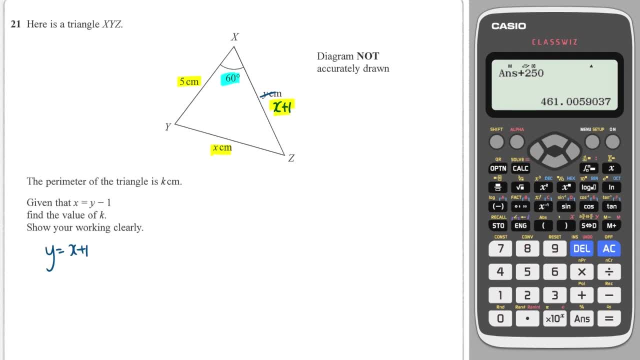 for each of the sides. so I'm going to use the cosine rule here and obviously the angle is capital A, which means this is little, a, which means these are B and C. so I would write that a squared is equal to B squared plus C squared minus. 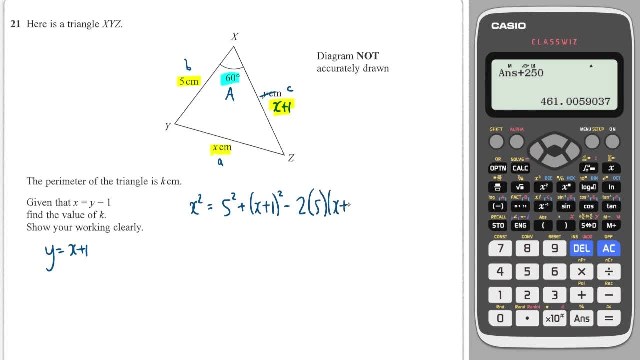 two lots of B C multiplied by cosine of the angle. okay, let's simplify. that's 25 X plus 1. all squared is x squared plus an X plus another X plus 1 times 1 is 1. I know that cosine of 60 is 1. 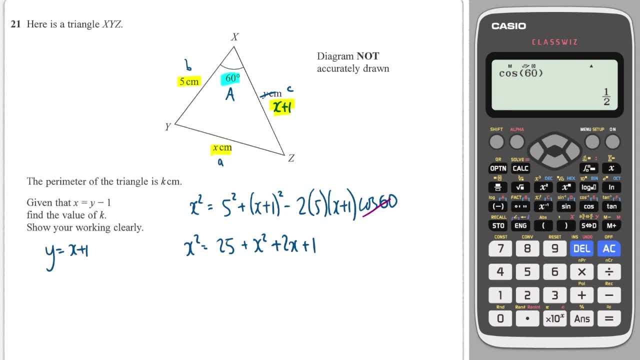 half, so I'm time link by a half and I'm Huntington by 2, so they were canceled. so this leaves me with minus 5 times x plus 1, and minus 5 x plus 1 is minus 5, minus, sorry, minus 5 x minus 5, so minus 5 x minus 5.